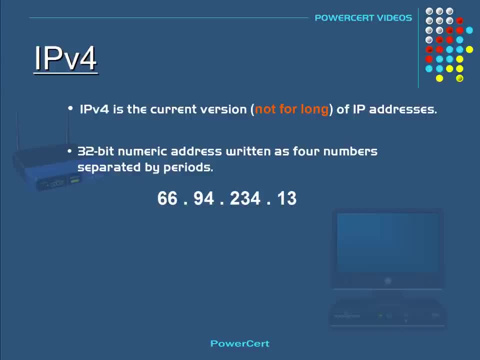 Each group of numbers that are separated by periods is called an octet. The number range in each octet is 0 to 255.. This address version can produce over four types of IP addresses. The IP address version can produce versions of over four billion unique addresses. 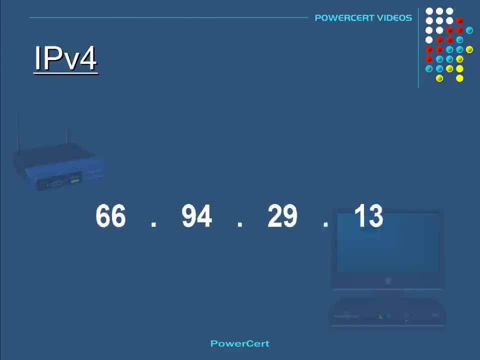 In the world of computers and networks, this IP address in this format here is meaningless. Computers and networks don't read IP addresses in this standard numeric format, and that's because they only understand numbers in a binary format. A binary format is a number that only uses hands and zeros. This kind of format型 is not suitable for non-numeric addresses. Shopify does not mean so. The binary format segmentation is another type of IP address reduction process which requiresrezion of international numbers in a global dashboard by aspects of IT technology and content transfer. hashtag3 and 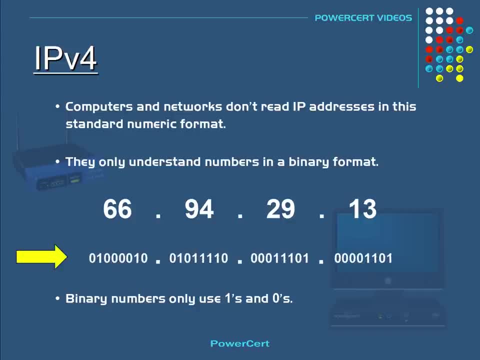 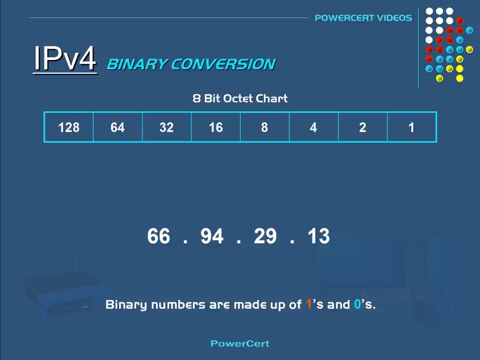 number for this IP address is this number shown here. This binary number is what computers and networking devices actually read. So the question is: how do we get this binary number from this IP address? IP address 4 is made up of four sets of eight binary bits, and these sets are: 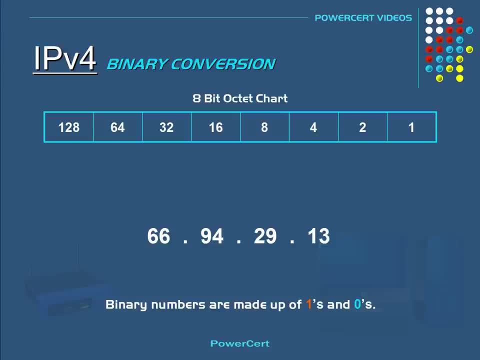 called octets. The bits in each octet are represented by a number. So, starting from the left, the first bit has a value of 128, then 64, then 32, and so on All the way down to 1.. Each bit on the octet can be either a 1 or a 0. If the number is a 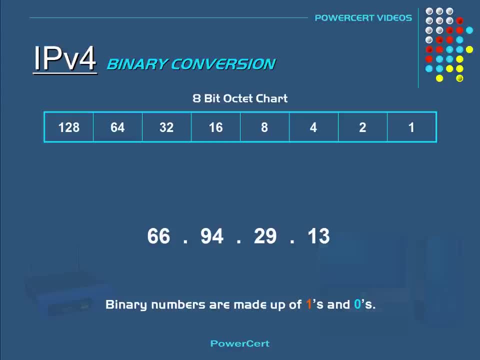 1,, then the number that it represents counts. If the number is a 0,, then the number that it represents does not count count. So by manipulating the ones and the zeros in the octet, you can come up with a range from 0 to. 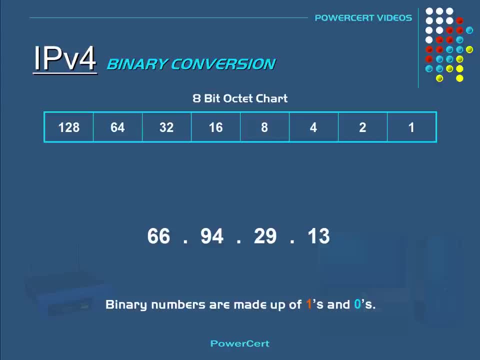 255.. So, for example, the first octet in this IP address is 66.. So how do we get a binary number out of 66? First you look at the octet chart and you would put ones under the numbers that would add up to the total of 66. So you would put a 1 in the 64 slot. So now you already have 64.. 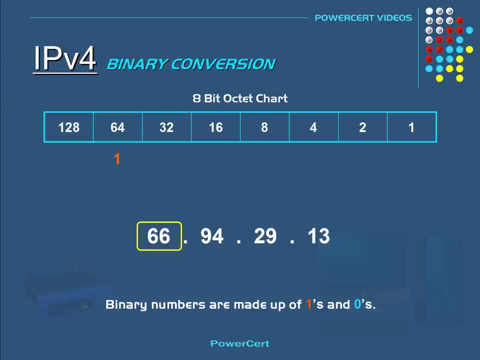 So we need two more. So let's put a number 1 in the 2 slot. So now, if we count all the numbers that we have ones underneath them, you would get a total of 66.. All of the other bits would be zeros. 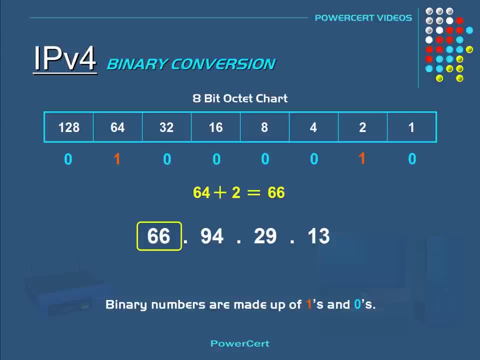 because we don't need to count them since we already have our number. So this number here is the binary bit. So we will do a 3 bit version of 66.. So we will put that number down here. So let's do the next number, which is 94.. So let's put a 1 under 64, 16, 8, 4 and 2.. So if we were to 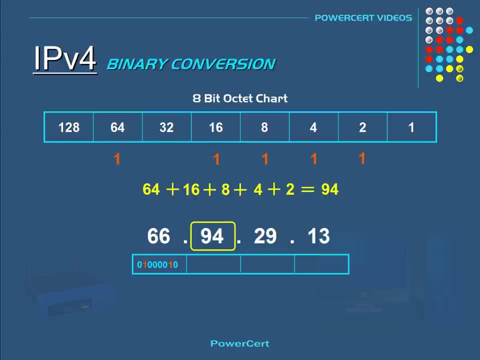 add all the numbers that we have ones underneath them, we would get a total of 94. And since we don't need that number, then we can just use what we have here. So let's go ahead and change the number. want to count any of the other numbers? we just put zeros under the rest. 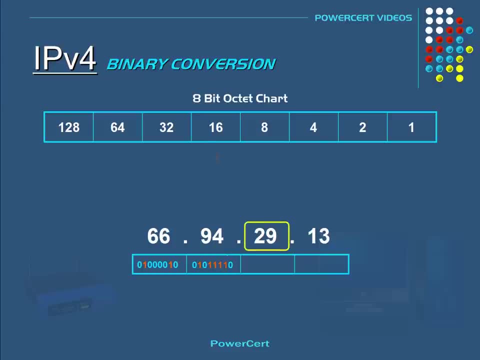 So the next number is 29.. So let's put a 1 under 16,, 8,, 4, and 1. And when you add all the numbers up, you get 29.. And our last number is 13.. So let's select 8,, 4,, 1. And when you add those up, you get 13.. 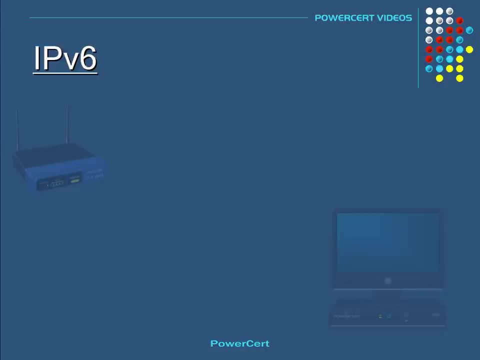 When the internet was first developed, programmers didn't realize how big it would become. They thought that IP version 4,, which produced over 4,000 gdy features, would work. billion addresses would be enough. but they were wrong. IP version 6 is the next. 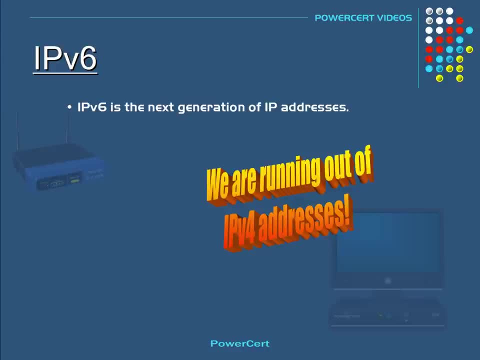 generation of IP addresses. The main difference between IP version 4 and IP version 6 is the length of the address. The IP version 4 address is a 32-bit numeric address, whereas IP version 6 is a 128-bit hexadecimal address. 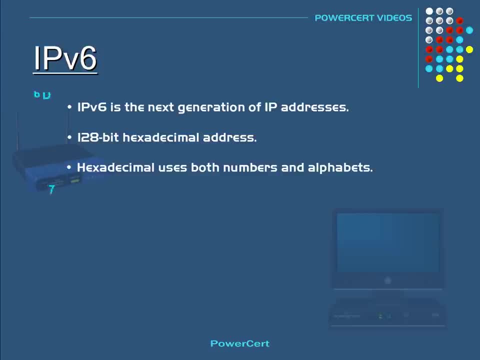 Hexadecimal uses both numbers and alphabets in the address. So with this type of address, IP version 6 can produce an unbelievable 340 undecillion IP addresses. That's the number 340 with 36 digits after it. So, as you might have, 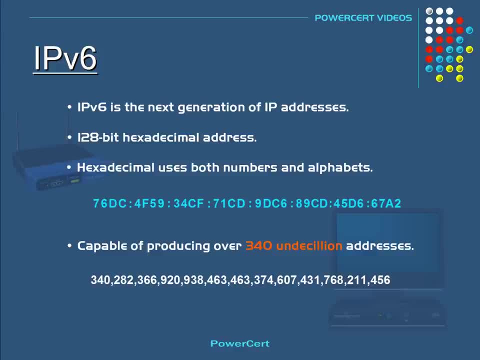 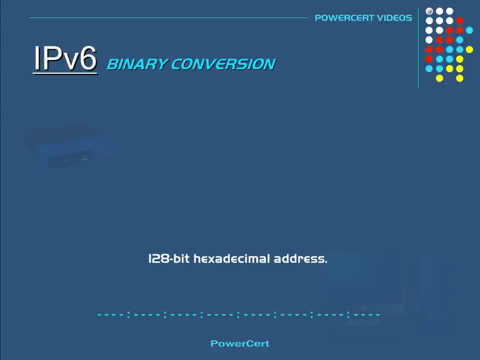 guessed, IP version 6 is more than enough for the foreseeable future. So, as stated before, IP version 6 is a 128-bit hexadecimal address. It's made up of eight sets of 16 bits, with the eight sets separated by colons, as you can see. 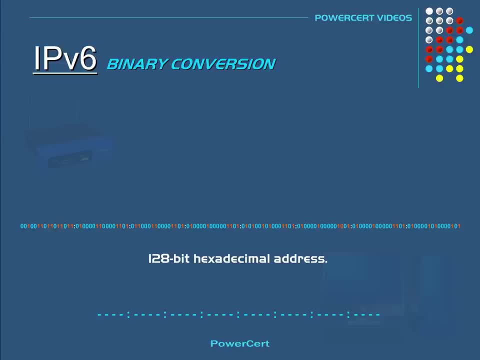 here. So in a similar way that we converted an IP version 4 address to a binary number, this is how we convert a binary number to a hexadecimal address. In an IP version 6 IP address, each hexadecimal character represents four bits, So we have to convert four bits at a time to get one hexadecimal character. 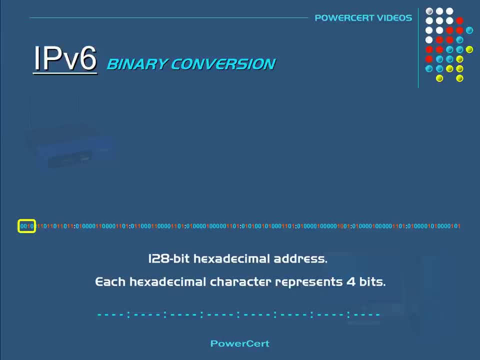 So, starting from the beginning, we convert the first four bits and put those bits up there against our four bit chart, which includes an 8,, 4,, 2 and a 1.. So if we count the numbers that we have ones underneath them, you wind up with a 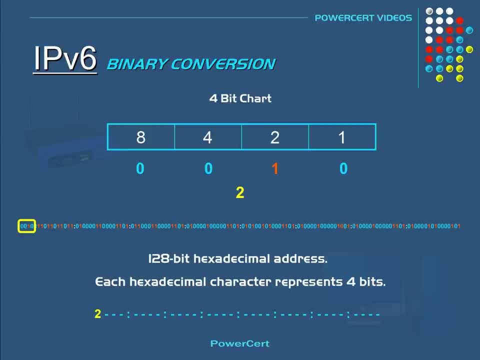 2.. So a 2 is the first hexadecimal character in this IP version 6 address. So let's do the next four bits and put those under our four bit chart. So if we count all the numbers that we have ones underneath them, we have a 4. 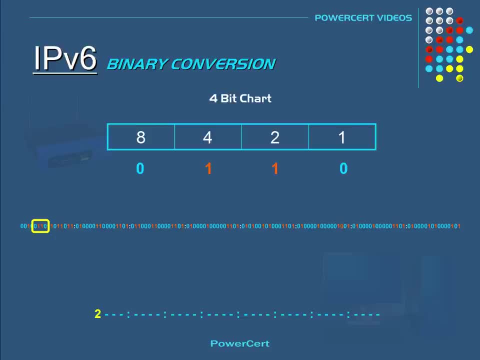 and a 2.. And if we add those up we get 6.. So a 6 is the second hexadecimal character in this IP address. So let's do our next set of four bits and if we add all the numbers that we have ones underneath them, we get a total of 13.. But the problem is, since 13 is a, 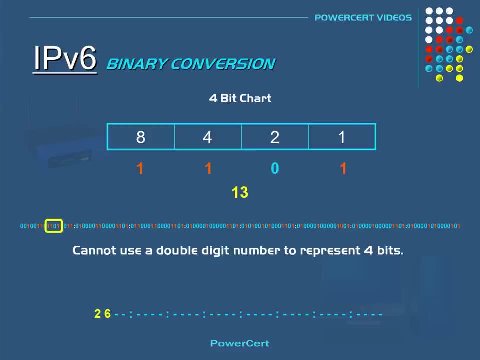 double digit number. we cannot use a double digit number to represent four bits, And that's because in a hexadecimal format double digit numbers have to be represented with a single alphabet, which is A through F. So in this case we have to use another chart for any four bits that the sum is 10 or higher. So in this